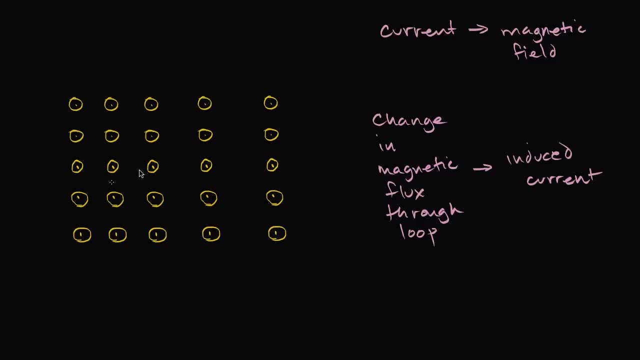 or at least that's what I'm trying to depict Now. if we did it with vectors, we would have bigger arrows pointing out over here than we would over there. But now let's do a loop of wire. Let me draw a loop of wire here. 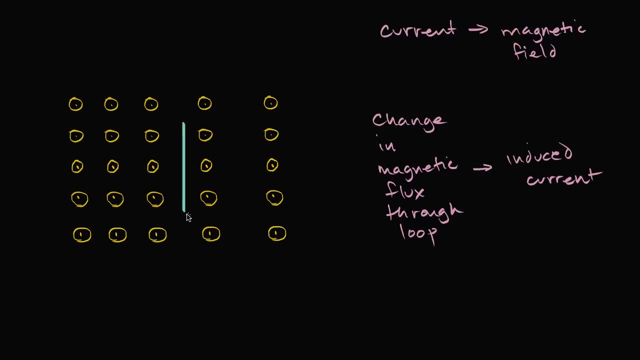 So let's say I have a loop of wire that is so, this is my loop of wire, My loop of wire. So if I just throw that loop of wire and if it's just stationary and it's in this magnetic field, 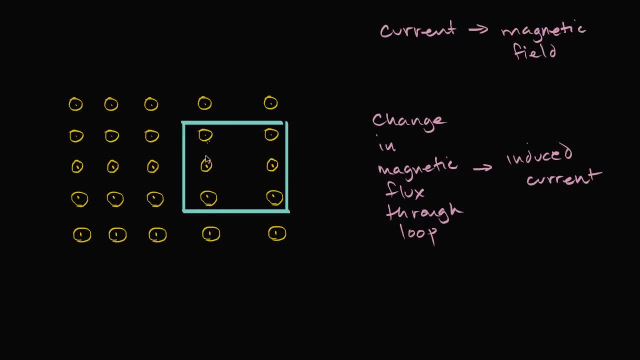 and the magnetic field isn't changing. I do have some flux going through the. I guess you could say the surface is being defined by this wire And if you're unfamiliar with the term magnetic flux, I encourage you to watch the video on magnetic flux. 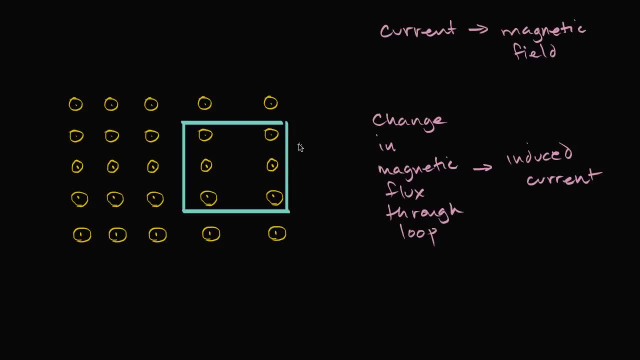 But if I just have this wire stationary in the magnetic field, nothing is going to happen. But I will be able to induce a current if I change the magnetic flux going through this surface in some way. So, for example, right now the magnetic field is pointing out of the screen. 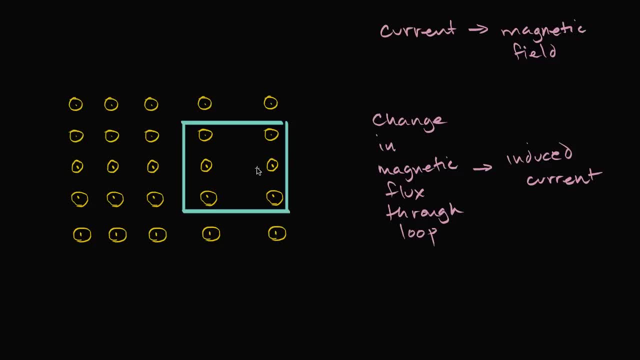 If I were to make it even stronger in the direction pointing out of the screen. so I guess one way to think about it is if I were to, if the change in the magnetic field, the change in the flux, were to get even stronger. 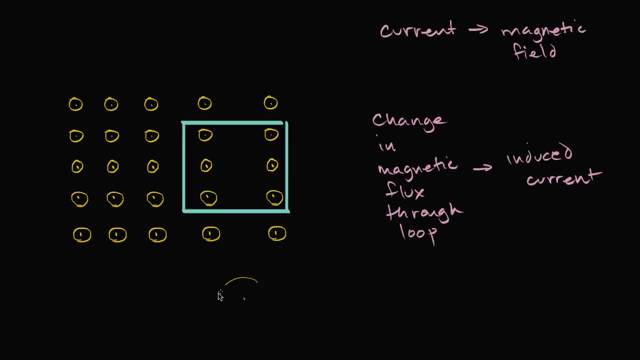 in the outward direction. so I don't know a good way to. so it's gonna get even stronger in the outward direction. I'll draw a big arrow there. I guess you could say that these things became even denser in this outward direction. 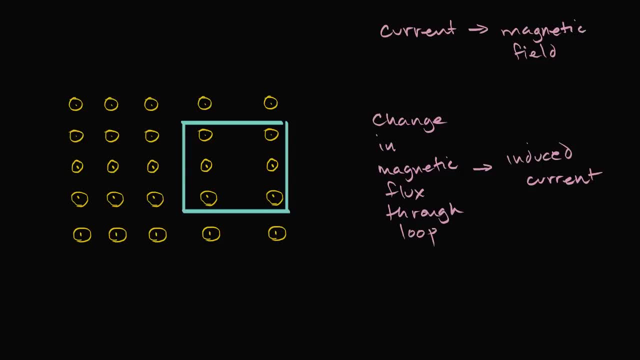 It is actually going to induce a current And the current that it will induce is going to go, is going to go in that direction. And let me draw a little bit clearer. The current is going to go in that direction. It's going to go in a clockwise direction around this. 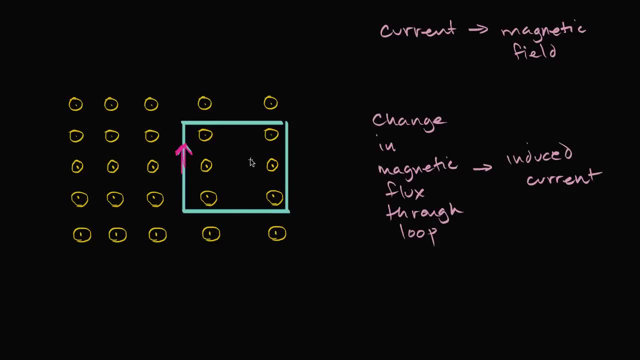 And that is because that change in the magnetic flux that induces a voltage, an electromotive force that causes this current to flow, That causes the current to flow. And there's other ways to change the magnetic flux. If I were to, if I were to lessen the magnetic field, 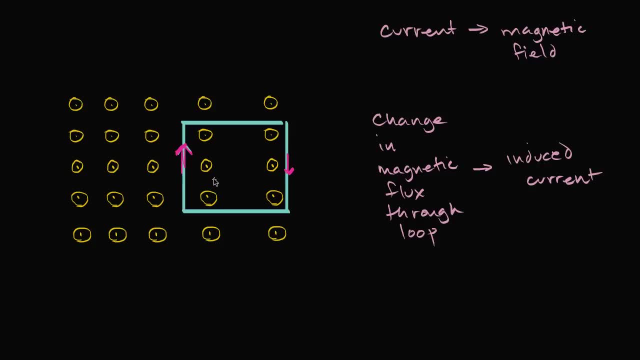 in the outward direction or another way. if the change in the magnetic field were inwards, then the current would go, it would go the other direction. But the key here is when I change the flux through this, through this surface defined by this wire. 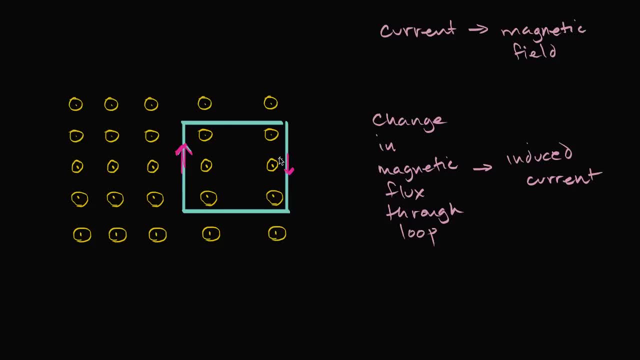 it's going to induce a current, The current isn't going to be there. if the thing is, if the magnetic field is stationary- and I'm not changing this, this, this loop, in any way- But as soon as I change the flux in some way, 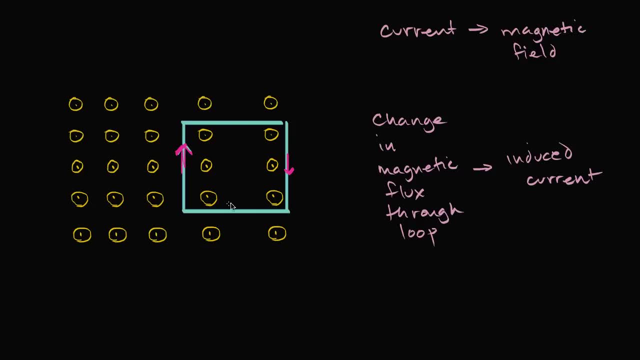 I am going to induce a current. I could also, instead of changing the field, I could actually move my. I could actually move my coil. I could move it that way. If I were to move it that way, the flux going through this surface. 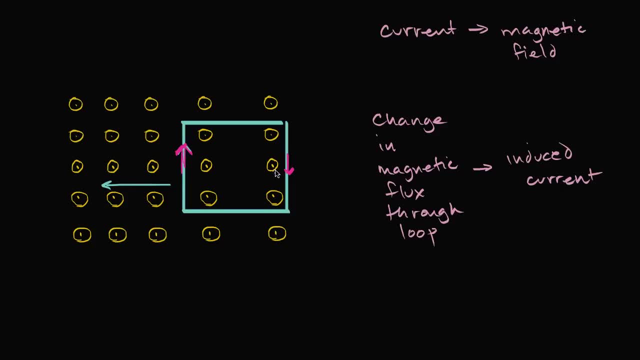 or I guess coming out of this surface will increase, Because if I move this to the left the magnetic field is denser. I guess it's stronger, So there'll be more flux through this area here. So if you move it that way, 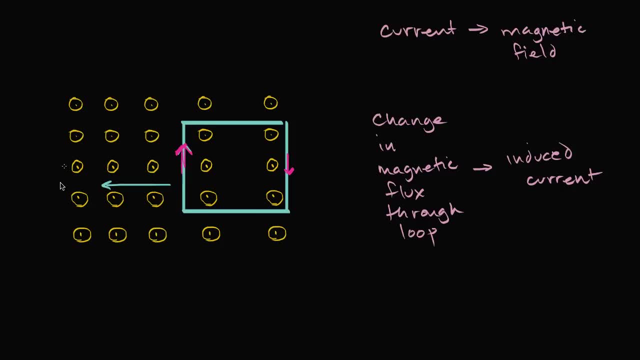 you also would have a current like this Now if you moved it the other way. if it was on the left-hand side and you moved it that way, it would also induce a current, But now, since the flux is lessening in the outward direction, 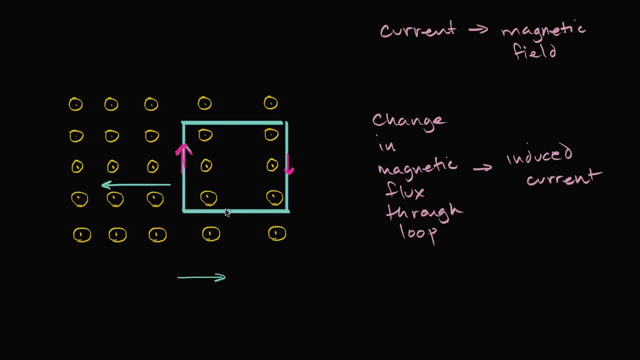 the current would go in the other way. Now there's other ways to change the flux. You could actually change the area of this actual loop If somehow it was made out of some- maybe- stretchy wire somehow, If you increased its, if you had increased 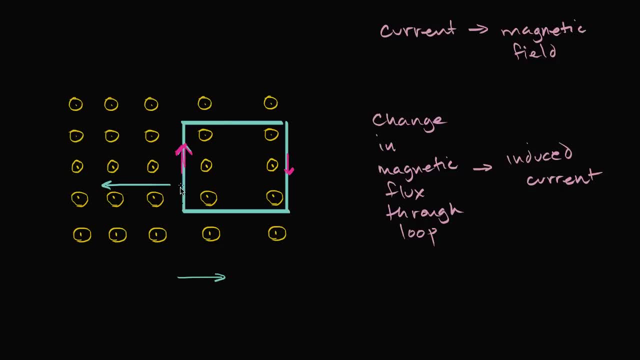 let me draw it this way: If you were somehow able to stretch it, stretch it so it contains, so the actual area increases. If you were able to stretch it out so that the actual area increases, which would cause the flux, the flux in the out-of-the-screen direction. 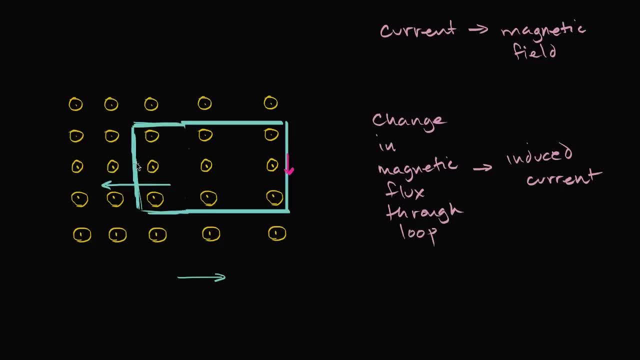 to increase even more. that also would induce. that also would induce the current, And so this whole idea of a change in magnetic flux inducing a current. this is the essence, and we'll go deeper into it in future videos. this is the essence of Faraday's Law. 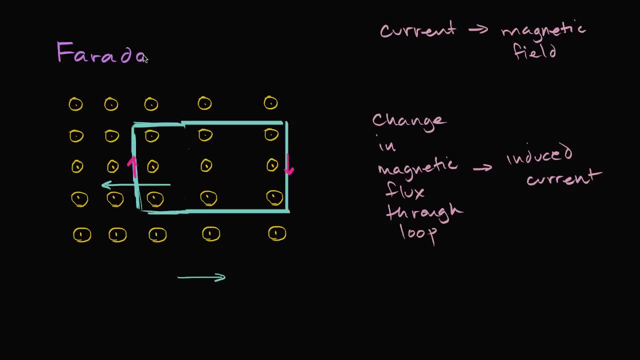 Faraday's, Faraday's, Faraday's Law, And we'll quantify this more in future videos. but it's just the notion that if I have a loop of wire and I have a changing magnetic flux through the loop of wire, that is going to induce a current in that wire.